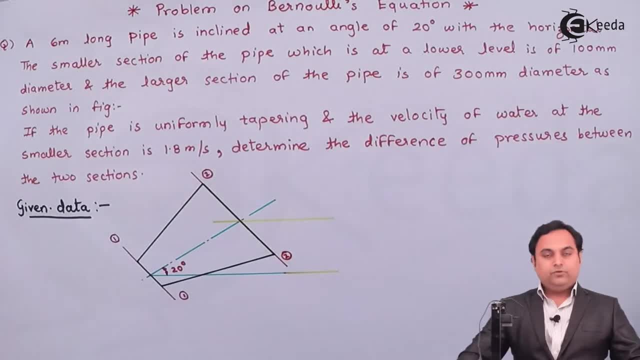 So here is the dippering pipe with, as given in the question, smaller section of the pipe which is at a lower level. So the smaller section- I have given it as section 1 1, at the lower level- is of 100 mm diameter and the larger section of the pipe is of 300 diameter, as shown in figure. 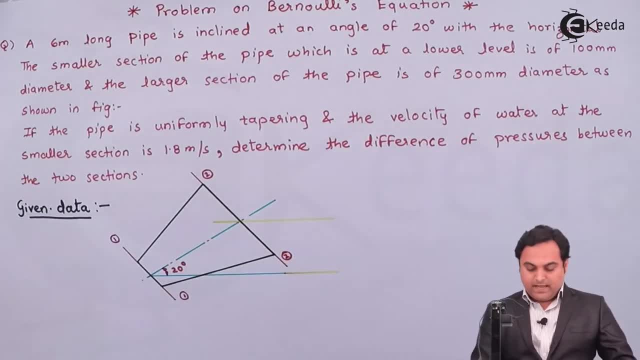 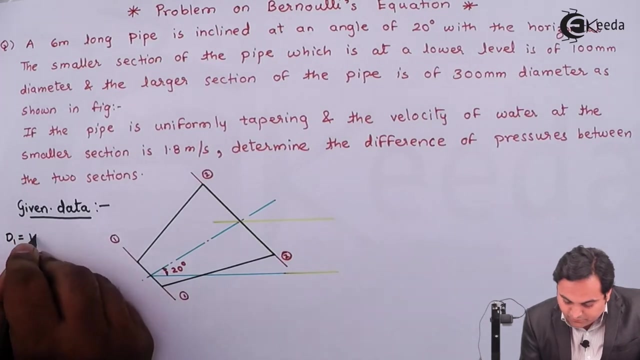 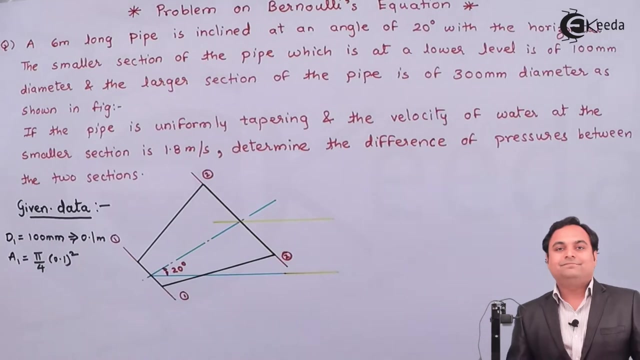 So here the diameter is 300 mm of the larger section and this pipe is inclined at an angle of 20 degree, as it is given. Now here I will mention the diameter D1, which is 100 mm of the smaller section, So it is 0.1 meter. then area 1 will be pi by 4 into 0.1 square and the value is 7.85. 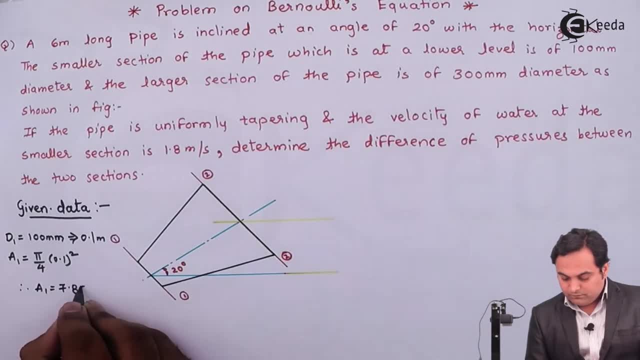 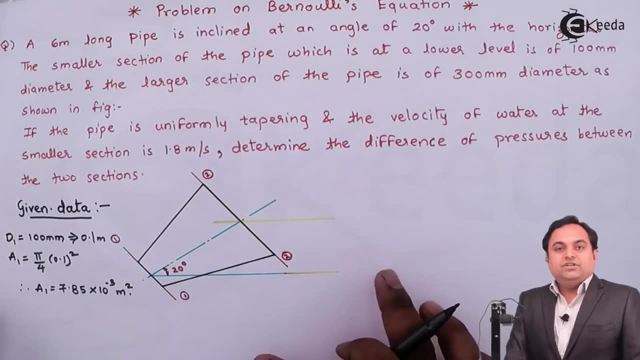 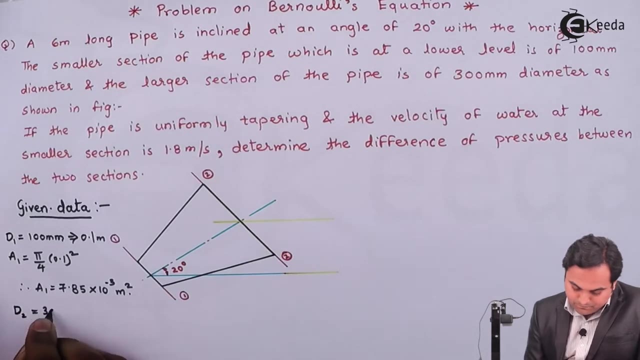 into 10 raise to minus 3 meter. square Diameter of the larger section is 300 mm. So this is the diameter of the pipe. Now for the diameter of the pipe Here I have given. the diameter of the pipe is 0.1 meter, as shown in figure. 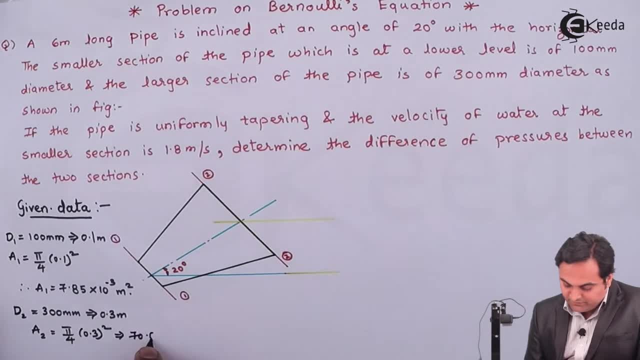 Area 2 is 70.69 into 10 raise to minus 3 meter square. Then it is given, if the pipe is uniformly tapering and the velocity of water, so the liquid given here is water and we know that. if it is water, then the density or mass density, 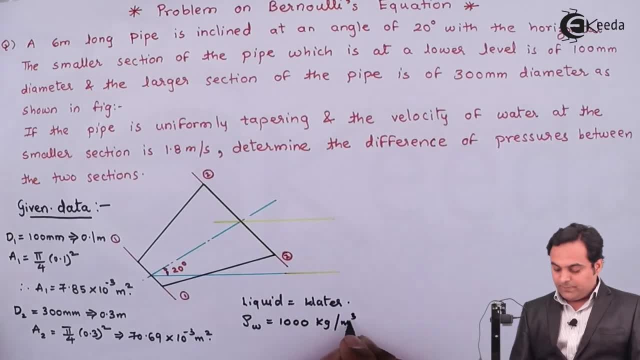 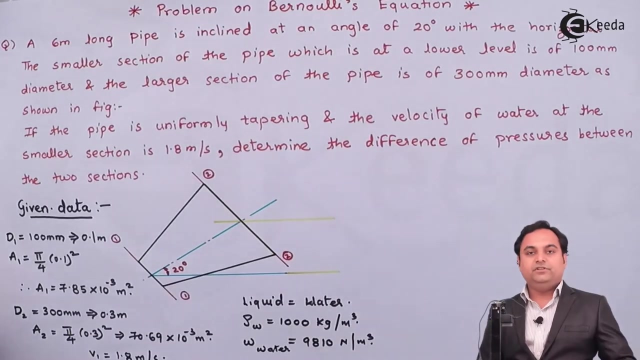 for water is 1000 kg per meter cube and the weight density of water is 9810 Newton per meter cube and the velocity at smaller section, that is, V1, is given 1.8 meter per second. We have to determine the difference of pressure between the two sections so that difference 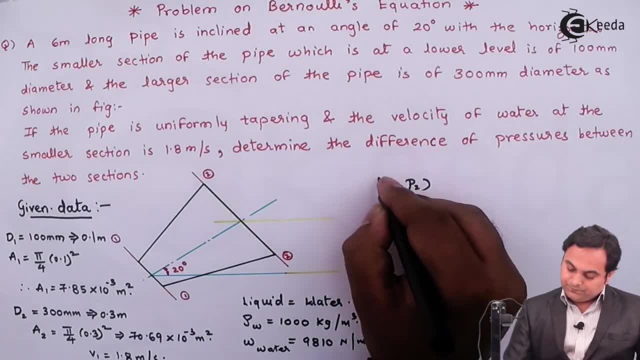 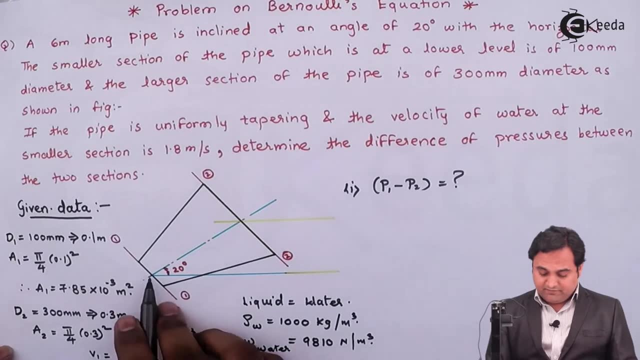 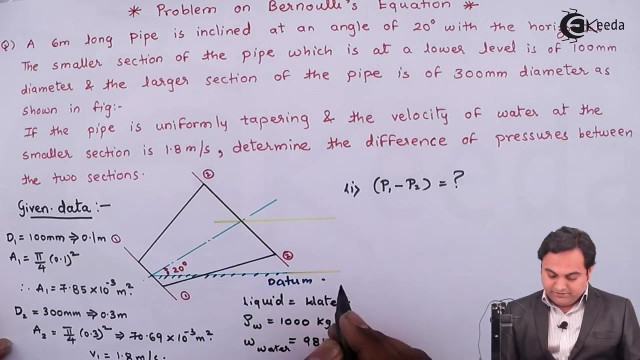 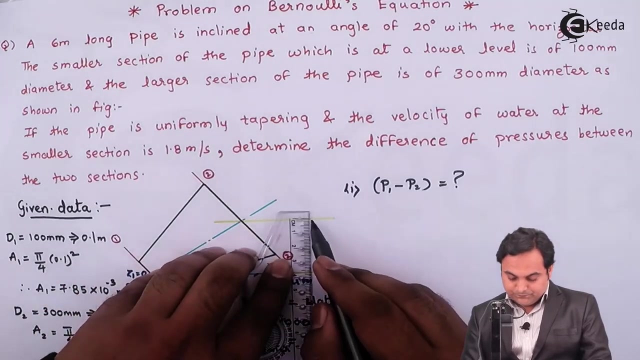 of pressure is given by P1 minus P2.. Now I will say that, since I would be taking this horizontal line as the datum or the reference, so this is the datum. So, from the datum, the height of section one Z1 is equal to zero and this is Z2.. 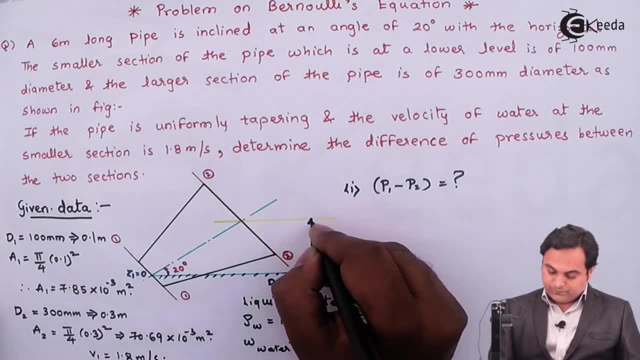 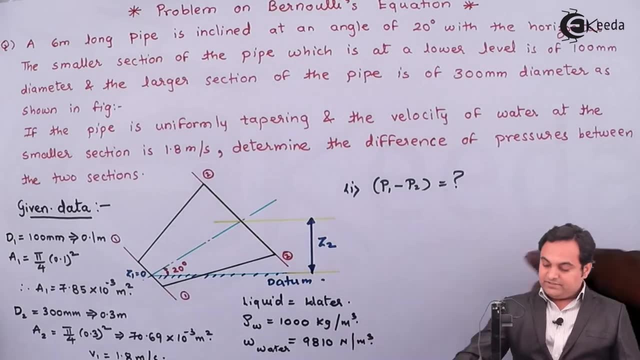 So we have to calculate the reference, So we have to calculate the reference, So this is the reference, So this is the reference, So this is the reference. the height of section second. so here I'll calculate this Z2 first into the. 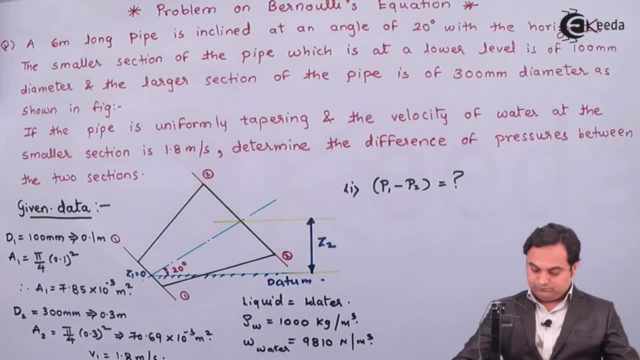 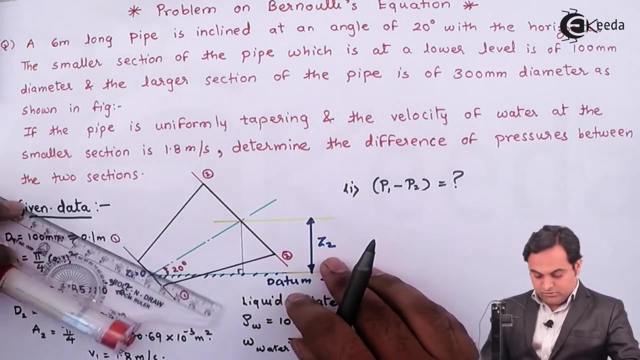 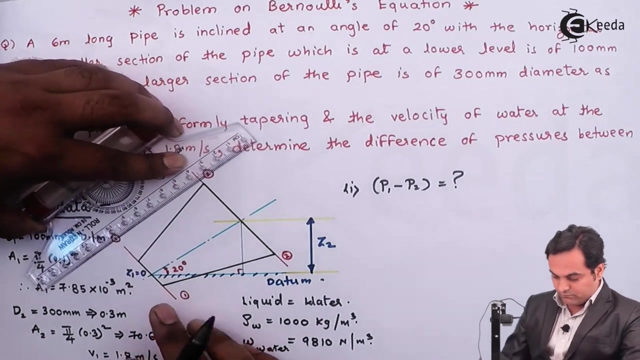 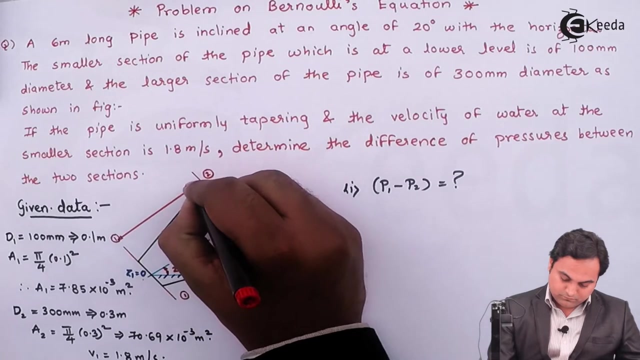 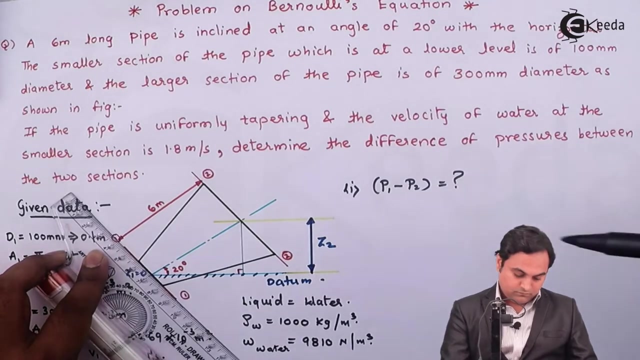 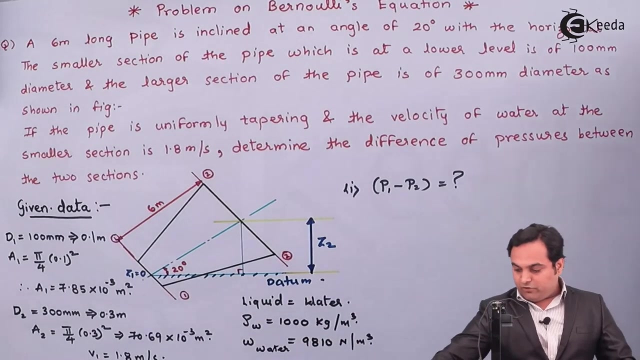 solution for that I'll drop a light vertical line. this angle is 90 and the length of the pipe is also there, and that length is given as 6 meter. so the tapering pipe is of 6 meter long. so here I can say that there is a right angle triangle which is formed here and 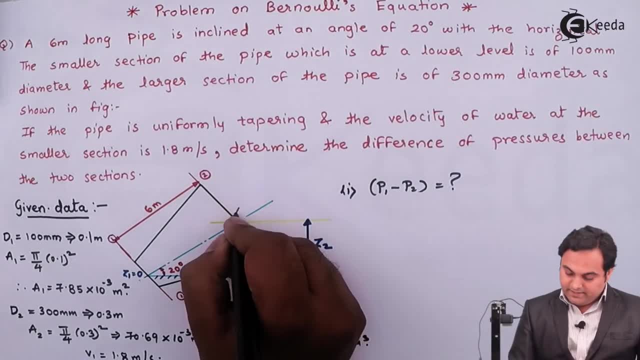 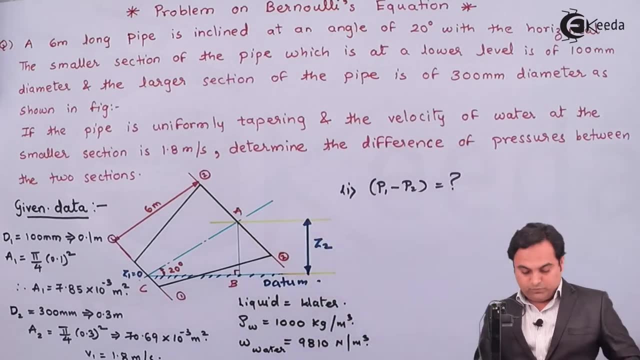 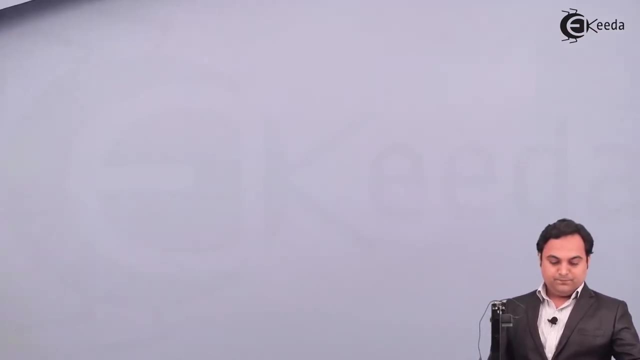 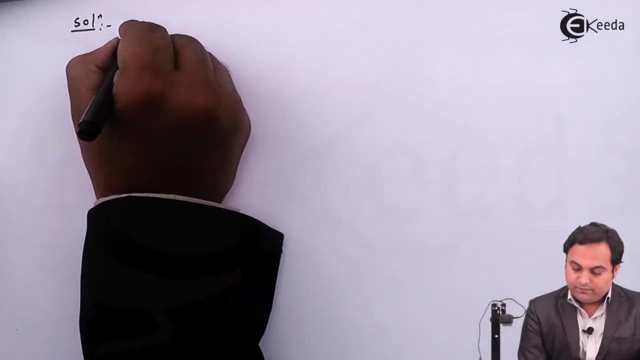 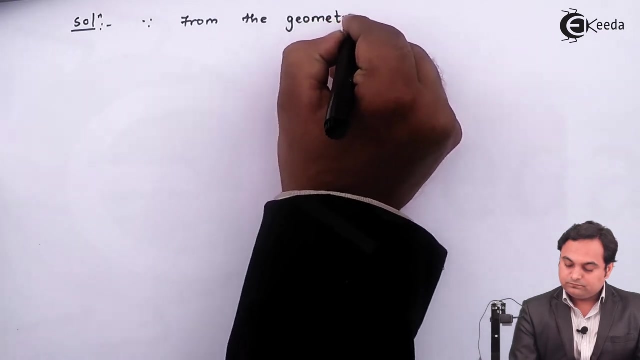 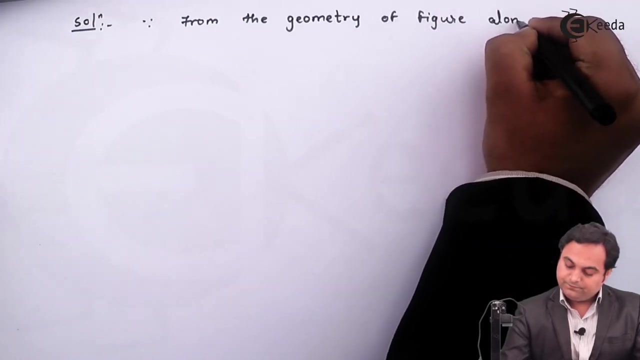 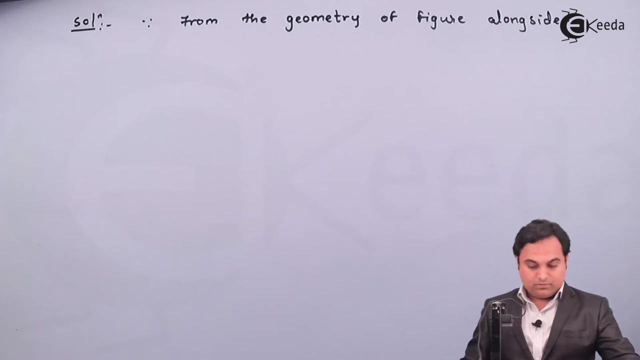 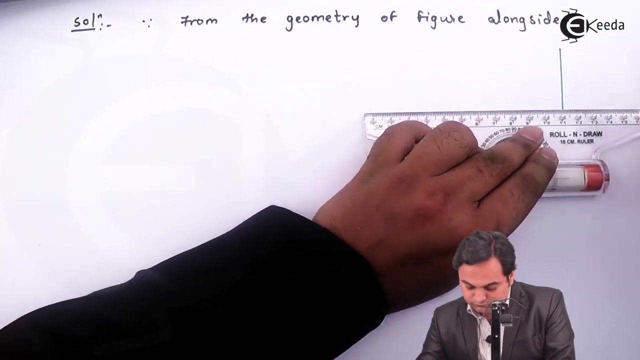 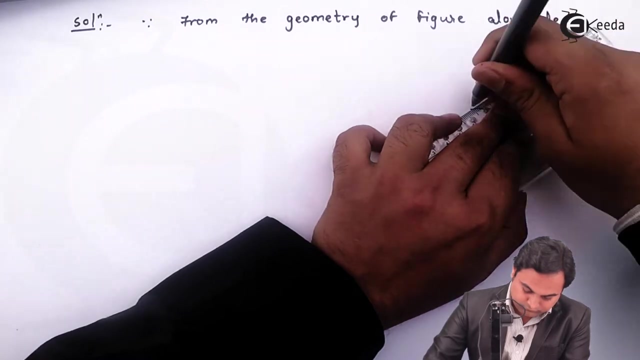 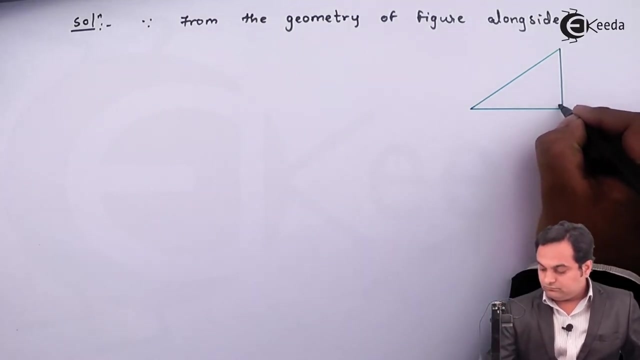 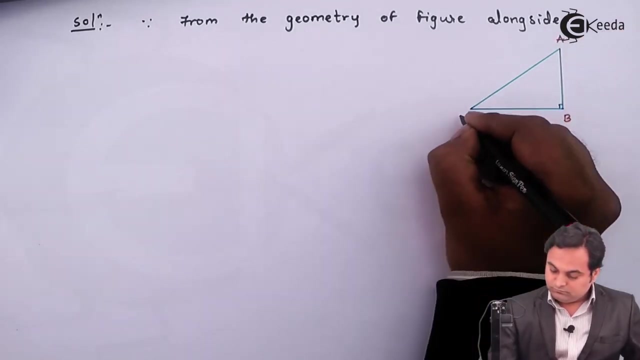 that right angle triangle. I'll denote it by ABC. now I need to calculate this height, AB, which is nothing but Z2. so, starting in this into the solution part, since from the geometry of figure alongside I'll draw the triangle ABC, here you, this is this, this is. 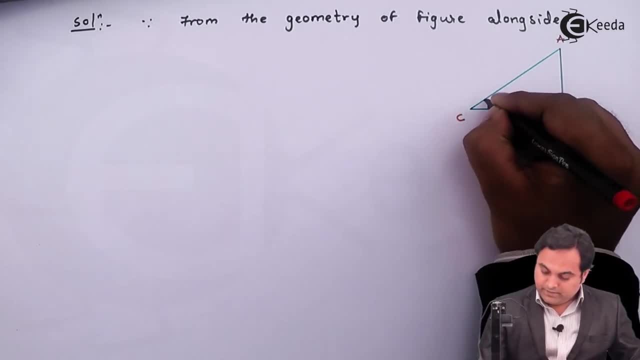 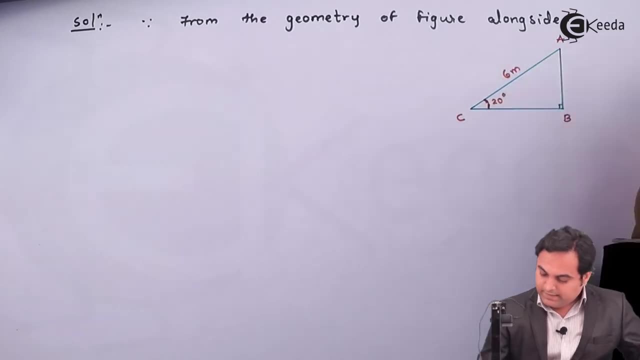 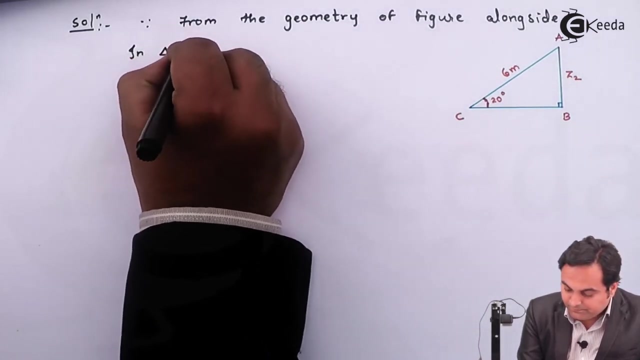 triangle ABC, the angle is 20 degree. AC is the length of the pipe, which is 6 meter, and this AB is Z2, what we have to calculate here. so I'll say that from the geometry of figure alongside in triangle ABC, sine 20 degree, that is. 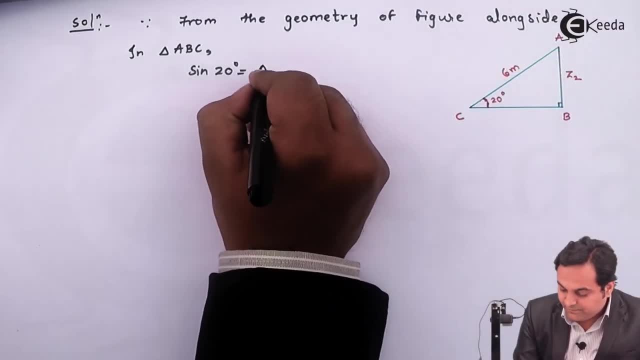 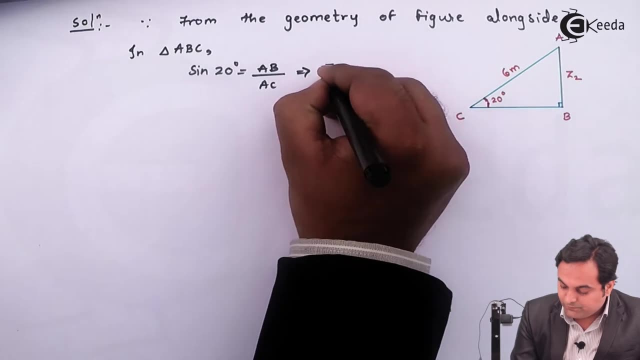 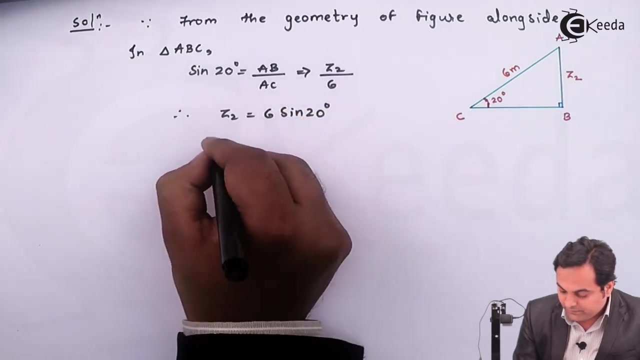 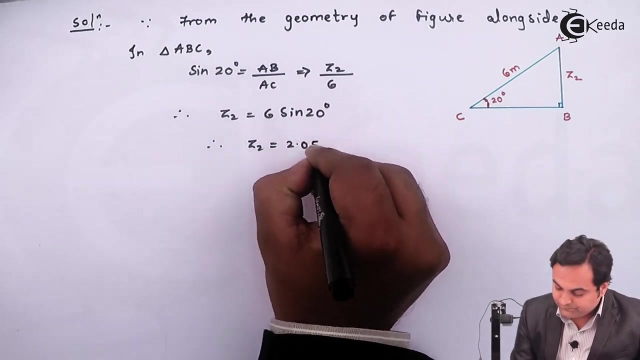 sine theta is equal to opposite side, which is AB, upon hyperdenous, which is AC. so AB is nothing but Z2, AC is 6, so therefore Z2 is 6 sine 20 degree, and hence my answer is: it comes out to be 2.05 meter. 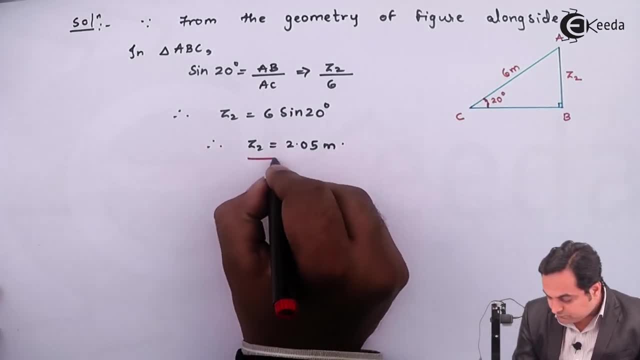 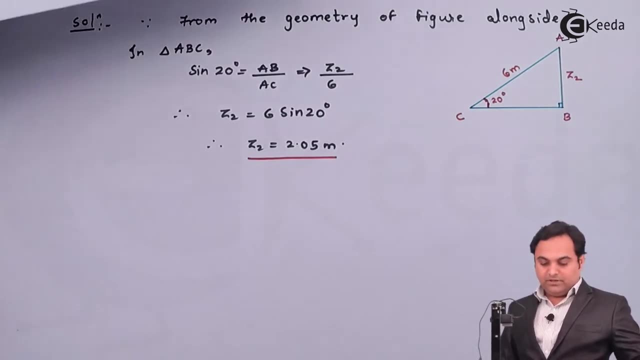 and hence my answer is: it comes out to be 2.05 meter, and hence my answer is: it comes out to be 2.05 meter after getting Z2, I would be applying Bernoulli's equation at section 1 & 2. after getting Z2, I would be applying Bernoulli's equation at section 1 & 2. 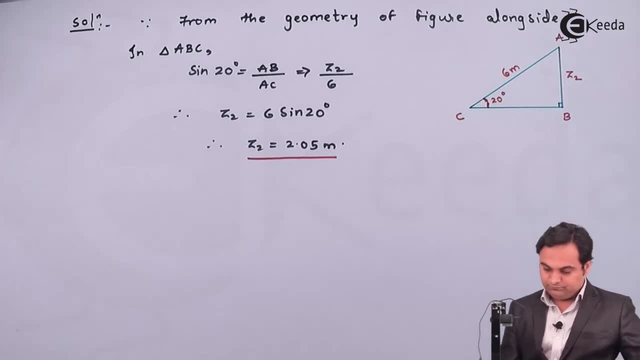 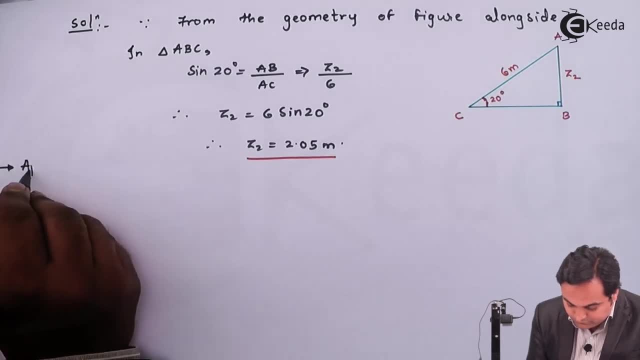 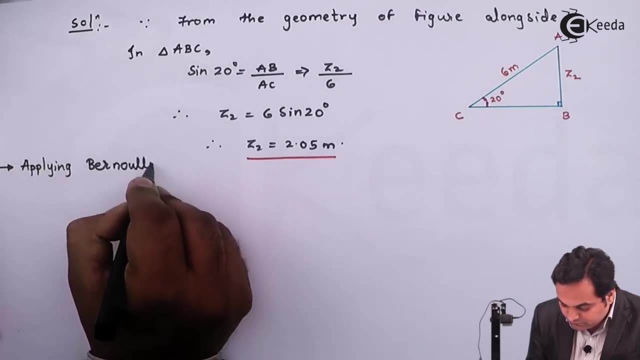 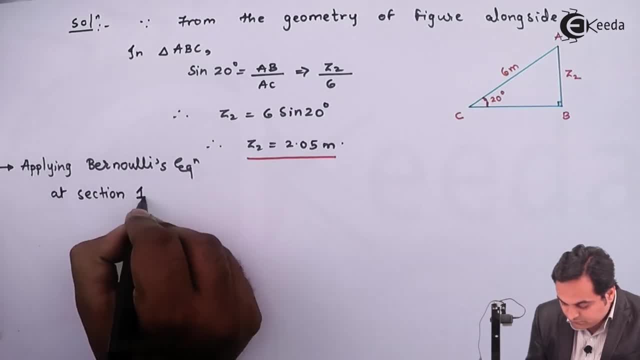 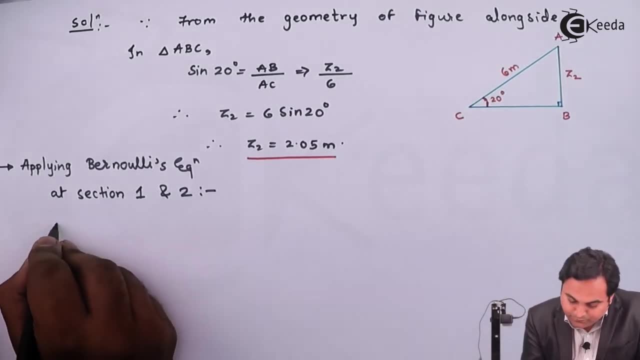 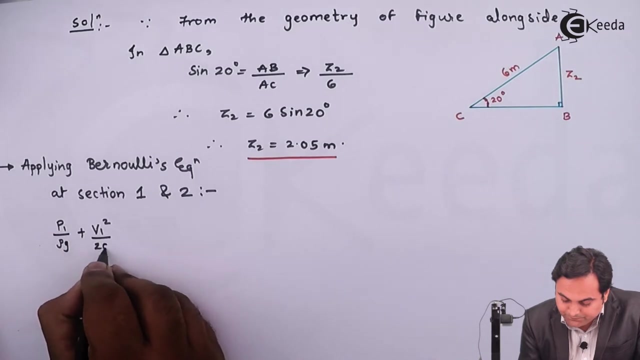 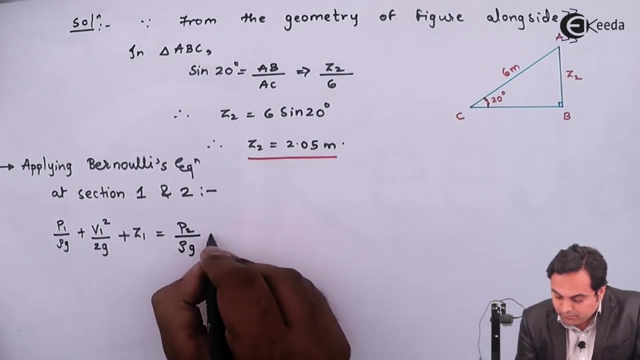 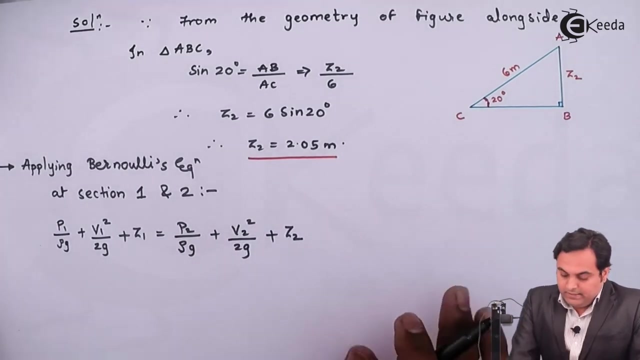 at section 1 and 2. so therefore it can be written as: p1 upon rho g plus v1 square by 2 g plus z1 is equal to p2 upon rho g plus v2 square by 2 g plus z2. and here in this case, since we want, 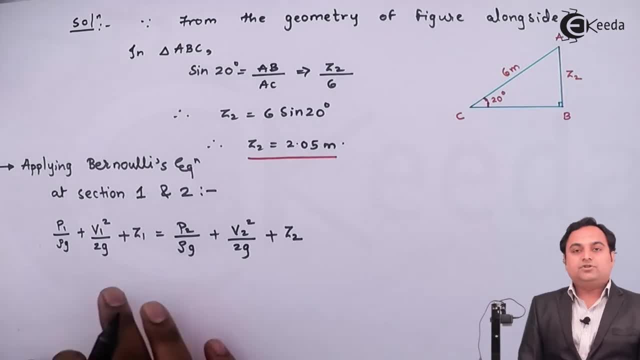 to calculate the difference in pressure. I will bring the pressures on one side. so it will be written as: therefore, when I bring p2 onto the other side, that that will be p1 minus p2, having the common denominator of p1 minus p2.. denominator rho g is equal to. here there is v2 square if I send v1 square onto the other side. 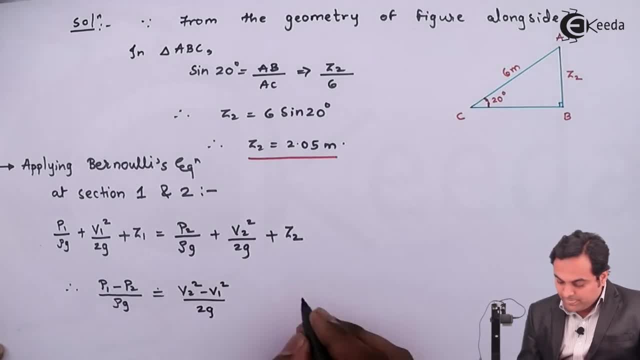 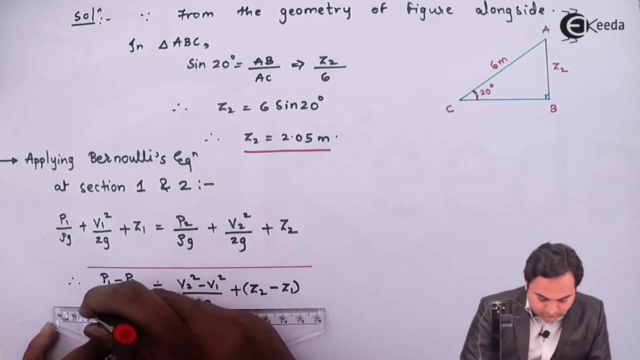 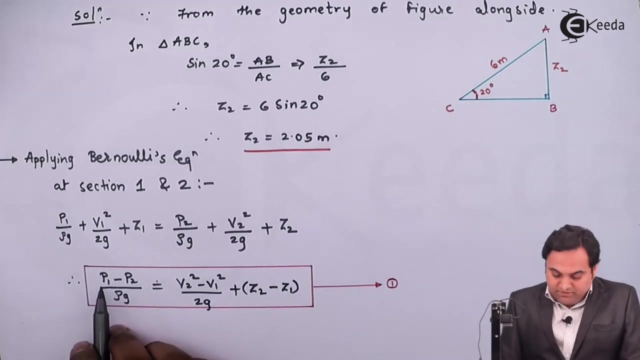 and then having the common denominator 2, g plus, here we have z2 if we send z1 onto the other side. so that is z2 minus z1. now I'll keep this as equation number first. now I'm keeping this as equation 1. so p1 minus p2 is what we have to calculate here. for that we 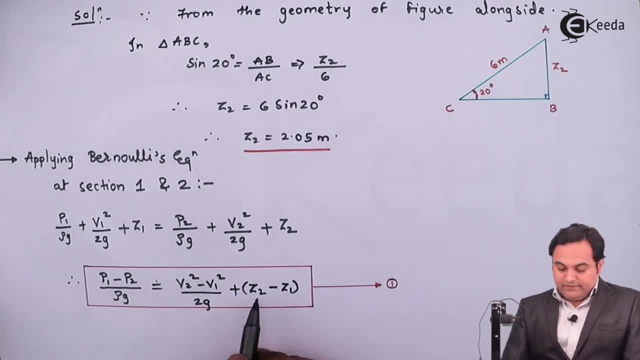 require v2, v1 and then z2 minus z1 g and the density they are constants. so here, if I see, v1 value is given in the problem, that is 1.8 meter per second, which is the velocity at the smaller section. v2 is what we have to find, that is the velocity at the larger section, and for that we 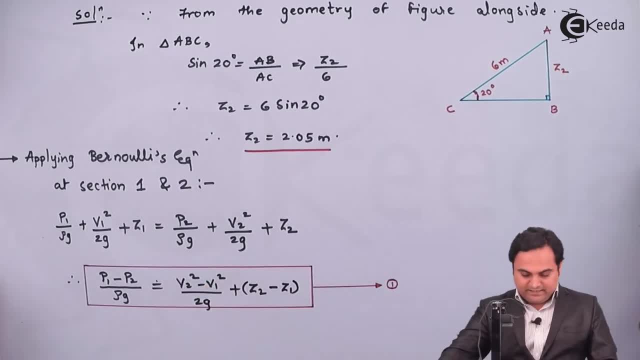 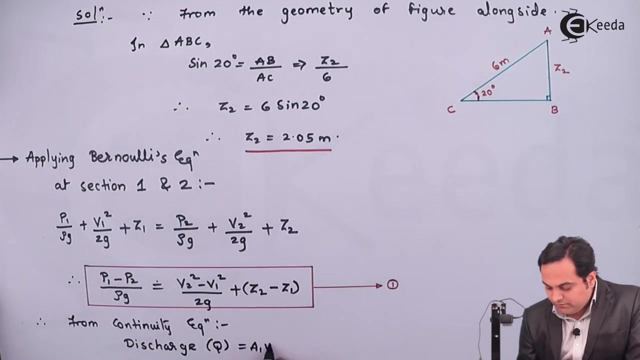 can easily use the continuity equation, so I'll say that after this. therefore, from continuity equation, discharge q is equal to a1, v1 is equal to a2- v2. so i will be using only this much part, because discharge is not known. a1- v1 is equal to a2- v2. 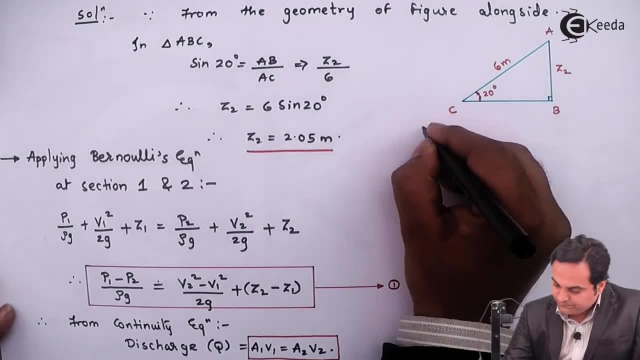 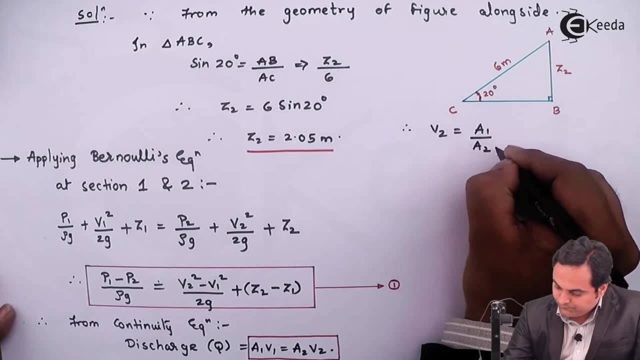 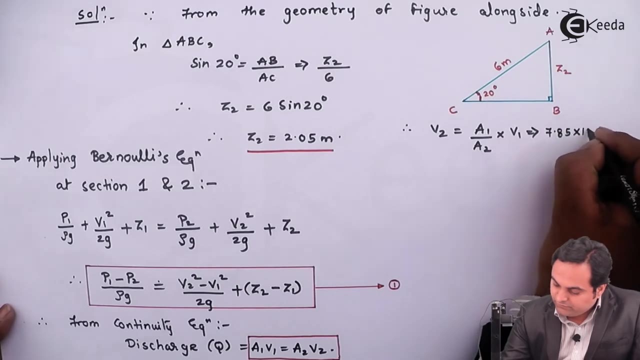 so from this i'll write v2 as therefore v2 will be equal to area 1 upon area 2 into v1. now area 1 is 7.85 into 10, raise to minus 3, area 2 is 70.69. 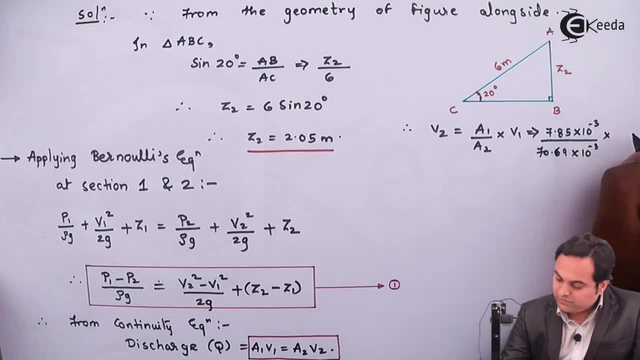 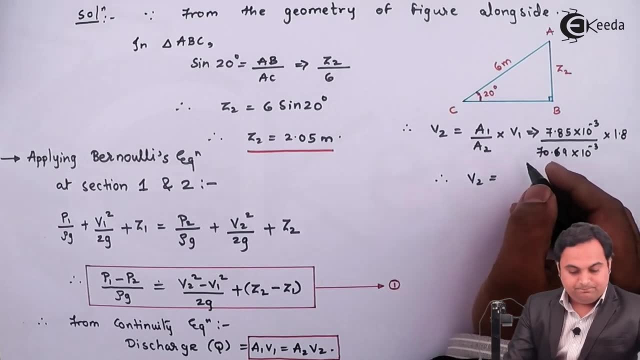 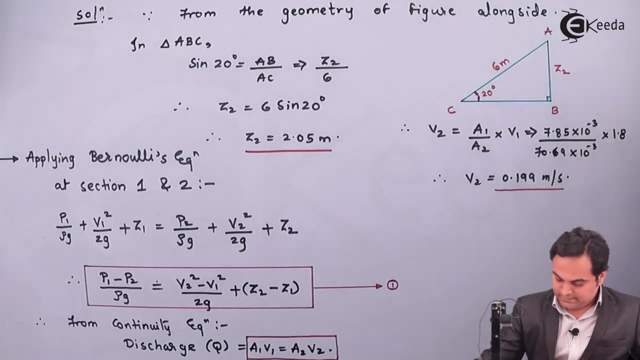 into 10, raise to minus 3 multiplied by v1 is 1.8. so from this i'll get v2 and my answer is it is 0.199 meter per second. so after getting v2 here, z2 is also known 2.05 and z1 is 0, as we see here. 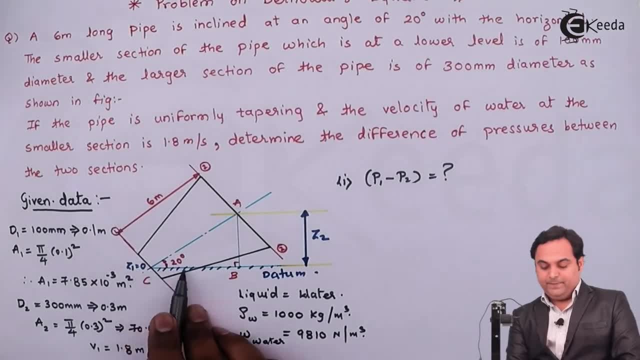 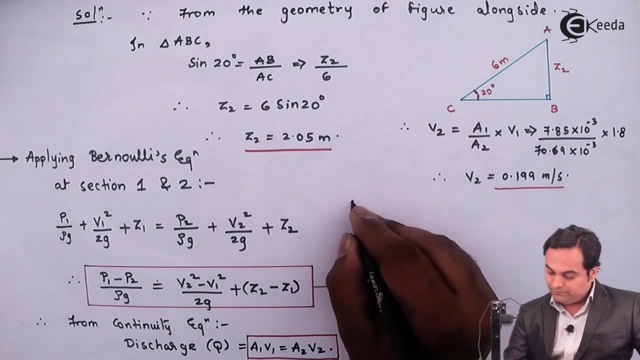 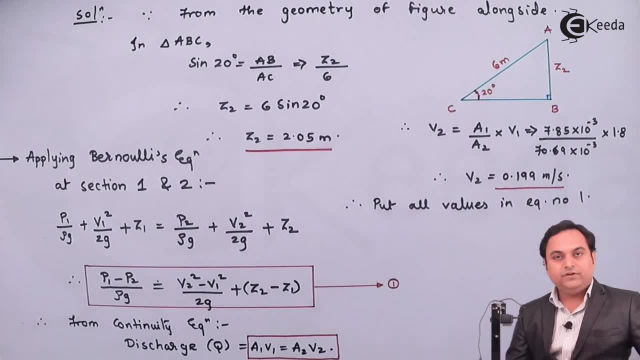 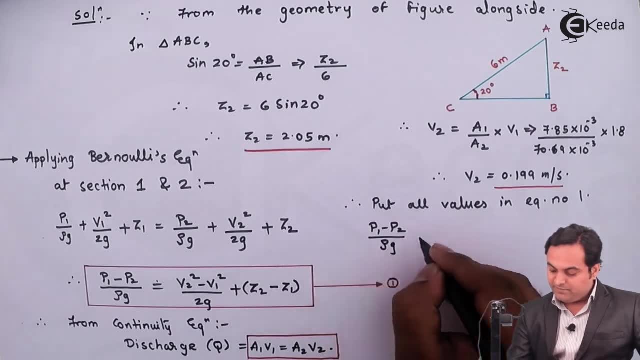 0.199 meter per second. put all values in equation 1, so we have p1 minus p2. i'll keep it on one side, rho g, for time being. i'm keeping as it is: velocity: v2: 0.199 square minus v1: 1.08. 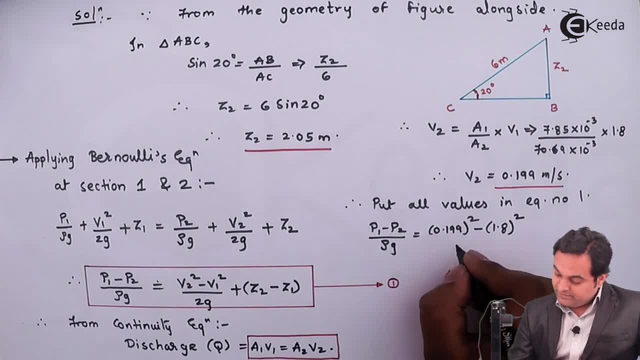 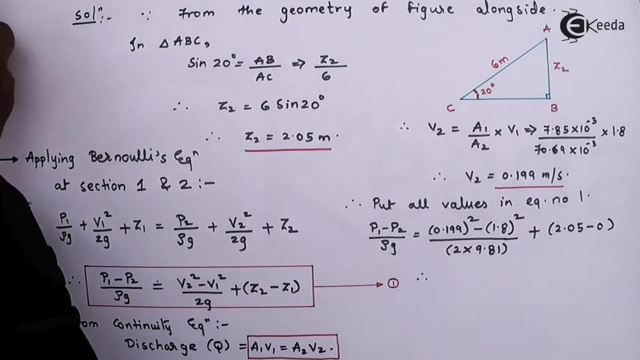 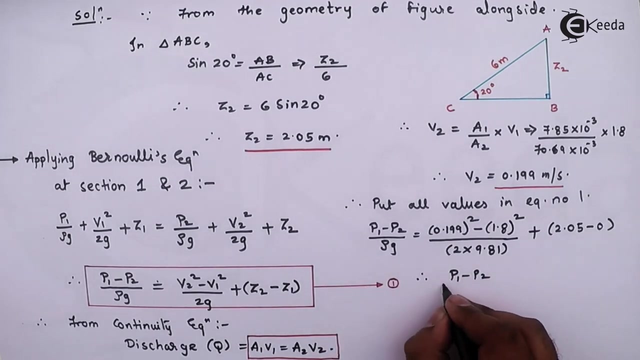 it is 1.8 square divided by 2g, that is 2 into 9.81, plus z2, minus z1. z2 is 2.05, z1 is 0. so therefore, when i reach up till here, and i'll say that p1 minus p2 upon rho g, which will be 9810, and these terms, 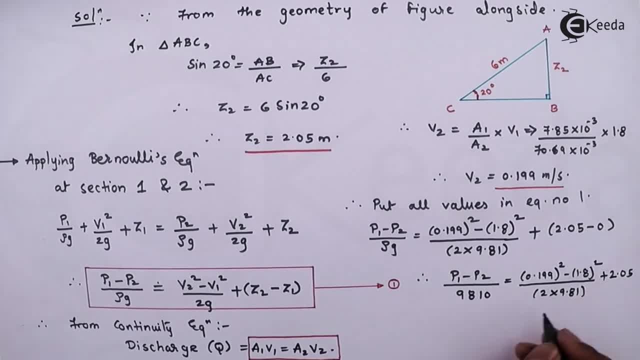 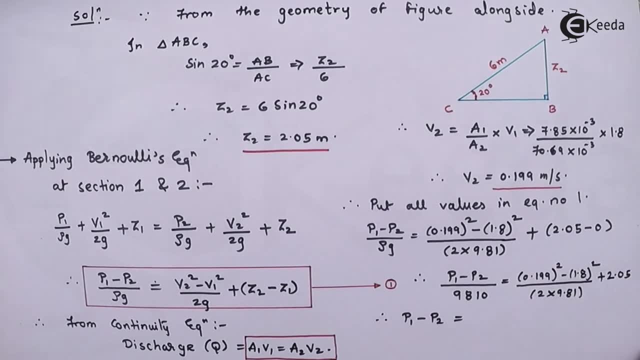 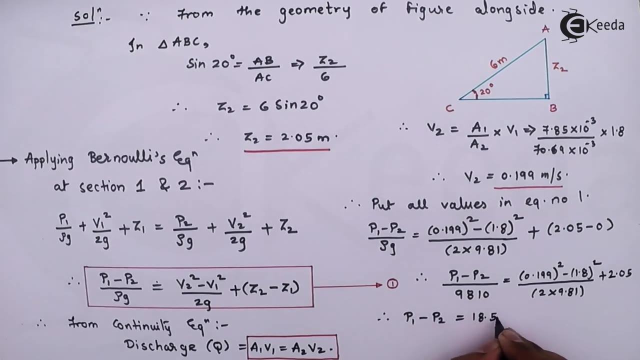 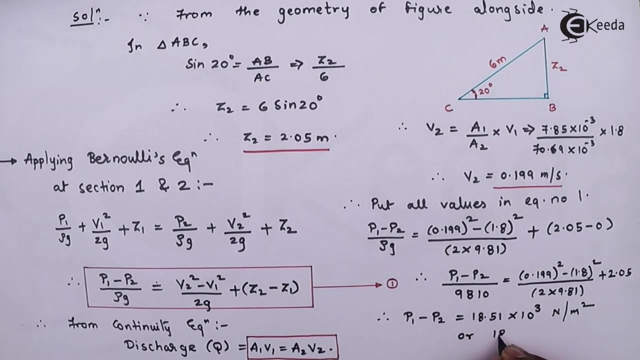 are equal to 0.199 meter per second. so if i calculate the right hand side, multiply 9810 onto the right hand side, i'll get my answer as 18.51 into 10, raised to 3 newton per meter square, or i'll say that is 18.51 kilopascal. 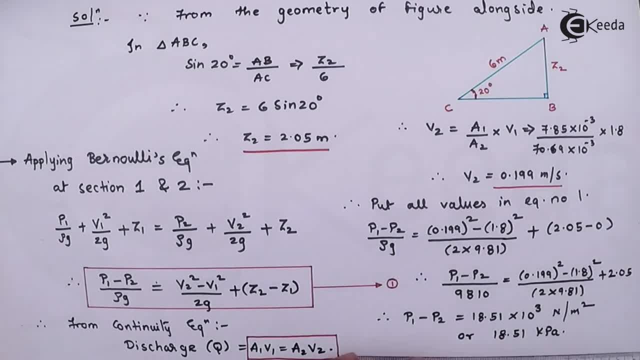 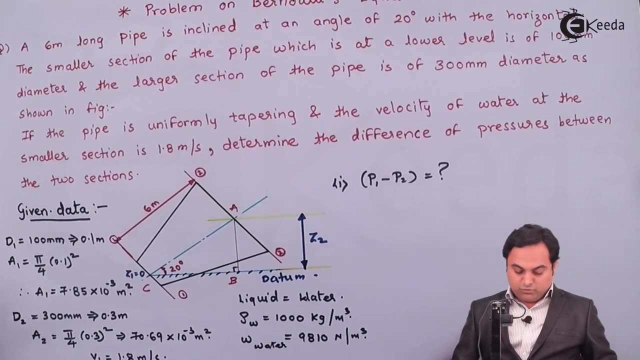 so it is our final answer, what we will answer in this second part. ok, so that's the final answer and we look when we look into the problem. it was only said that determine the difference of pressure between the two sections. so i can say the difference of